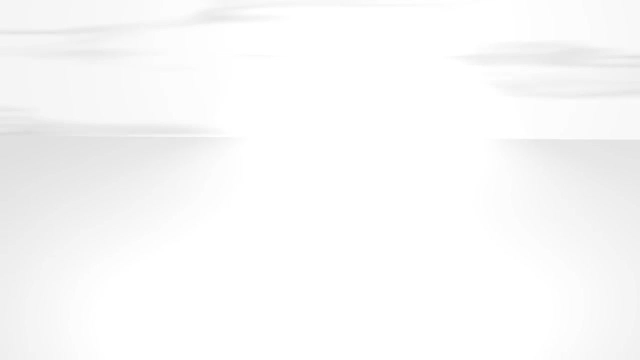 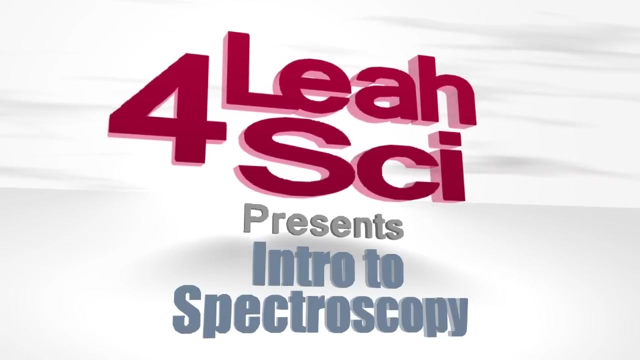 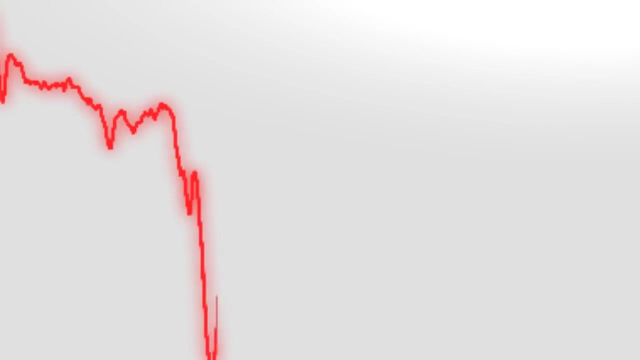 Leah here from leah4scicom, and in this video I will give you a quick introduction to the different types of spectroscopy that you will encounter in the standard organic chemistry course. While I will not go into the specific graph interpretation details, I will show. 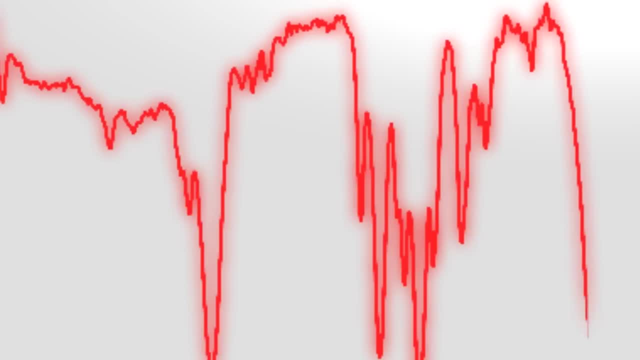 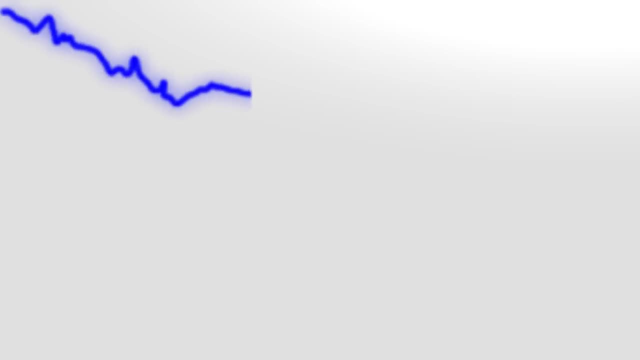 you when and how to use the information given so that you can come up with an educated guess to identify the molecule in question. And the best part is- and don't tell anyone I said this- is that you don't really have to understand the mechanics or what is happening. 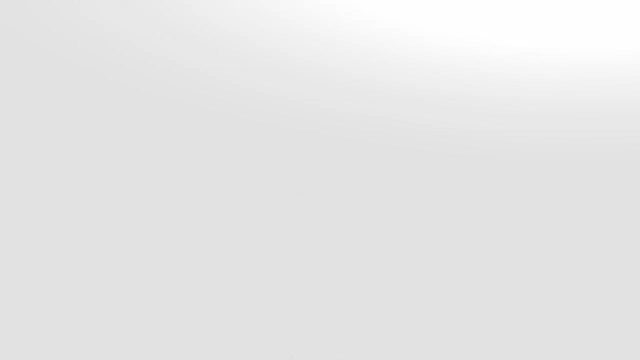 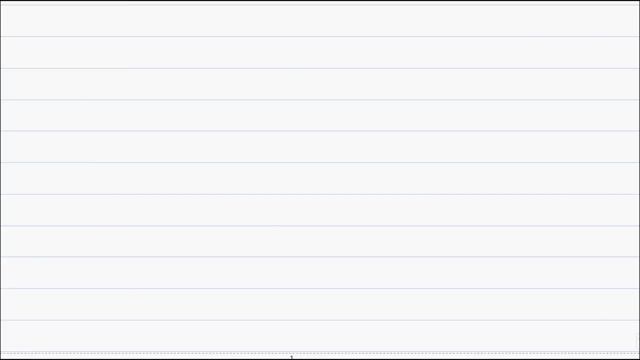 within the type of spectroscopy. As long as you know how to read and interpret the graphs, you should be okay doing these types of problems. The most common type of spectroscopy problem you will come across, and my favorite, is NMR. NMR stands for Nuclear Magnetic Resonance. There are two types of NMR spectroscopy that 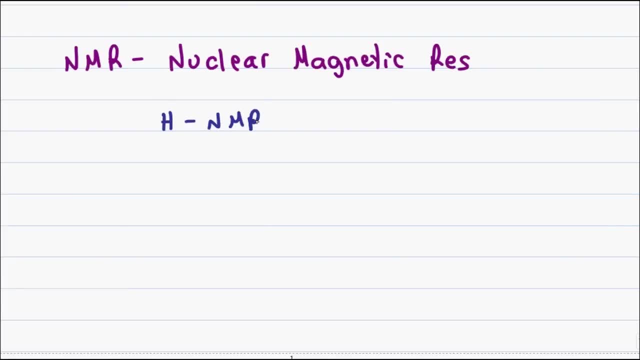 you will be studying. The first is H-NMR and the second is C-NMR. When given a C-NMR spectrum, analyze it in terms of what type of carbon atoms you have and potentially, how many carbons. That's all you need to see from carbon NMR, H-NMR, if given on your practice. 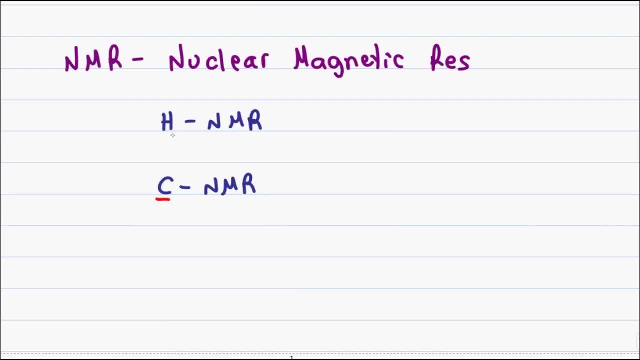 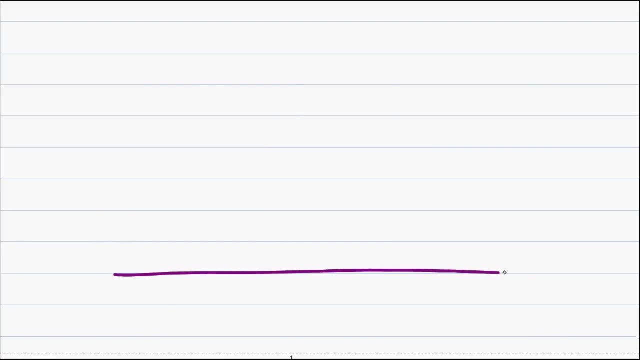 problem will essentially give you the entire story of the molecule. It gives you the relationship between the hydrogen atoms, What atoms they are attached to and, in turn, how these different groups relate to each other. Your H-NMR graph will show up with numbers ranging from 0 to 13 and you will 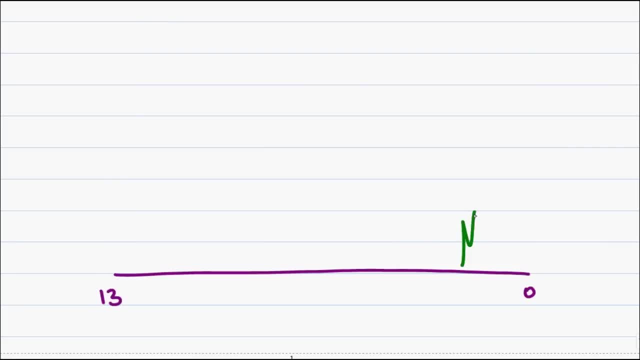 have peaks of various sizes and shapes, So let's draw in some random ones for now, and yes, I will go through how to analyze these in a future video. At first glance, these look scary. However, there are many things you can deduce from. 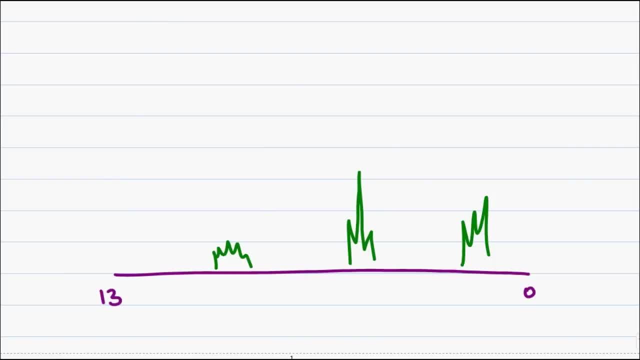 these peaks, if you understand it, including the types of atoms that are attached to them. First, the number of hydrogens within the neighboring molecule and how the different pieces fit together with each other. You will likely be given a table with numbers, but don't. 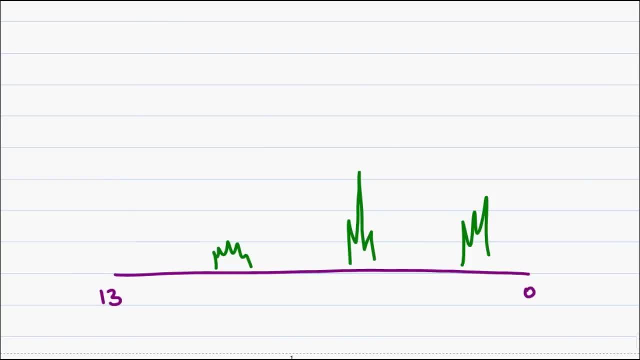 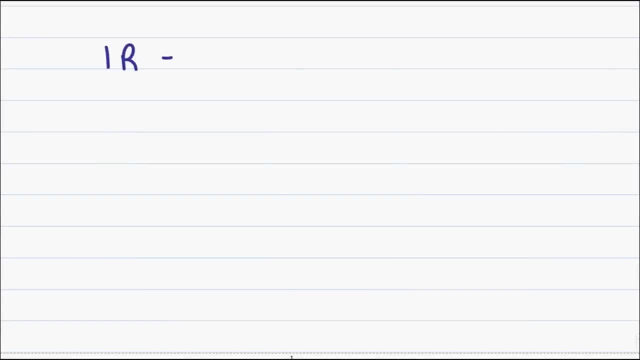 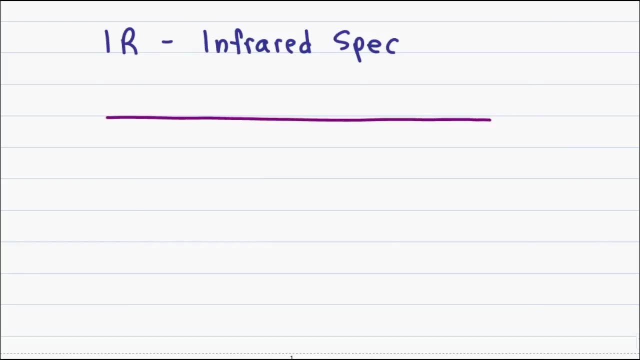 memorize them Instead, study and try to understand the different peaks, where they show up and what they mean in the molecule. Another common graph that you will see is the IR graph, or infrared spectroscopy. The graph for IR will range from the numbers between 0 and approximately. 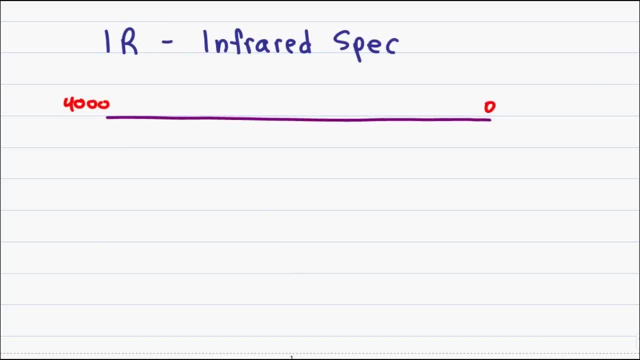 4000.. Within this graph you will see many different upside down hills, valleys and just peaks overall. Unlike NMR, with IR you cannot look at the graph and definitively say this applies to this specific group or this specific molecule. However, if you are given IR in a problem, 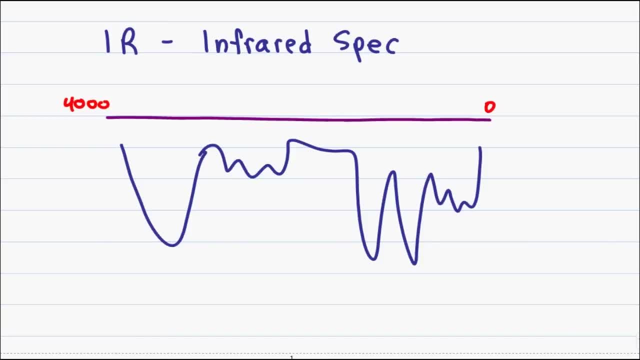 this is very useful for identifying functional groups. Just like with NMR, you will be given a table of values and descriptions of the bands that you will find. Don't memorize them. Instead, analyze them on a graph and learn to recognize the different. 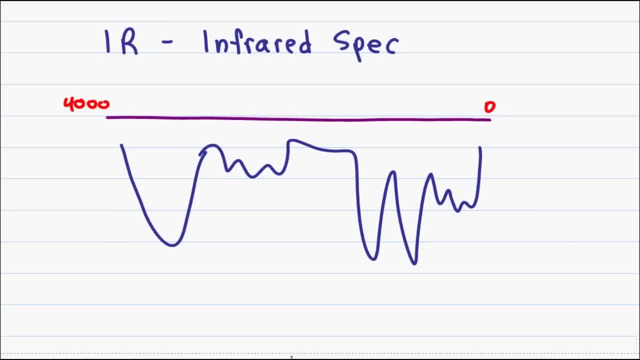 bands where they show up and how they show up in relation to other ones. IR will typically be given in a problem together with something like mass spec or NMR, and you can use these two graphs in conjunction to help come up with a molecule. 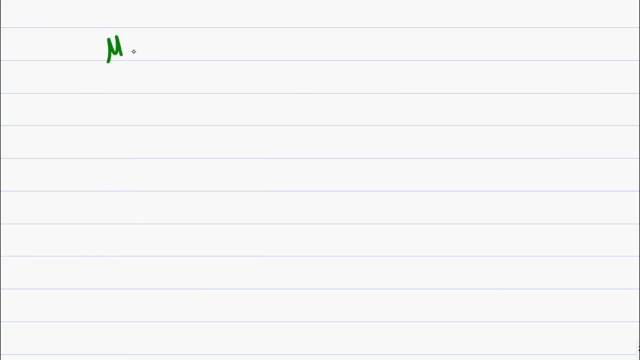 Another very useful and hard to read graph is going to be mass spec or mass spectroscopy. This graph shows you how, when a molecule is broken down, what the different fragments look like. Some students will analyze mass spec and panic because they cannot put the pieces together. However, this is not what I want you to focus on. 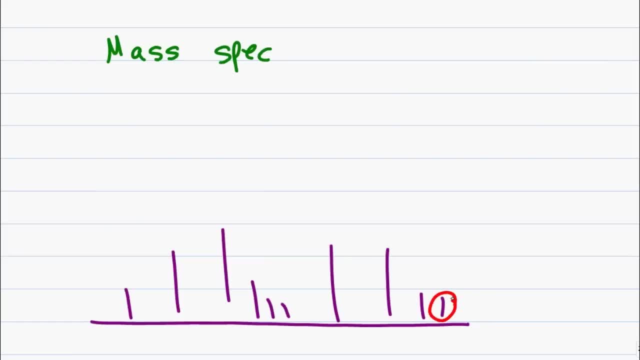 What you want to look for in your mass spec is your highest number, which gives you the molecular weight of your molecule, and this ultimately helps you find the molecular formula. One more thing that mass spec is very useful for is helping you identify specific atoms within your molecule, such as a branch, For example. if you have a branch in your high. 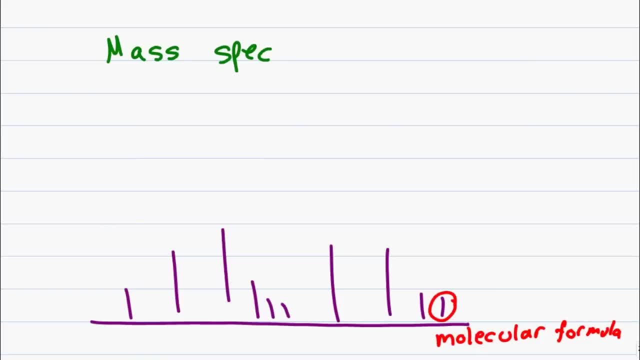 molecules such as a bromine or a chlorine atom. While you can go into more detail to try to analyze the fragments to see what your molecule is, don't waste your time on this. instead, just take your formula, go to your NMR, try to put the molecule together. go. 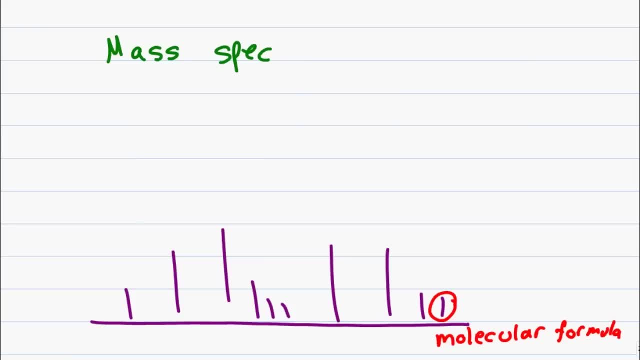 to your IR, try to find your functional groups and using all of them together you should be able to come up with a decent molecular formula and molecular structure. In future videos I will break down the analysis of the different spectroscopy and walk you through a few problems to help you understand. but the purpose of this video is just to give